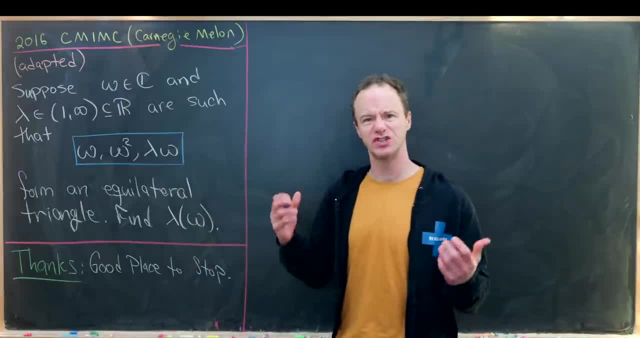 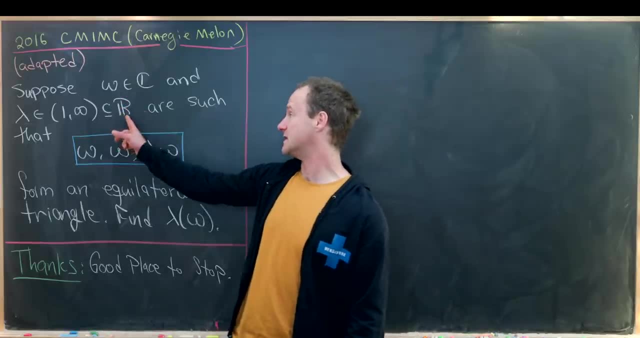 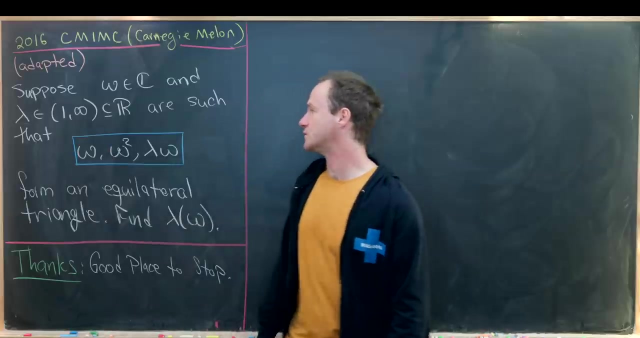 And I've also adapted this problem a little bit to generalize it. So let's suppose that omega is a complex number and lambda is a real number which is strictly greater than 1. So in other words, it's on this interval from 1 to infinity. 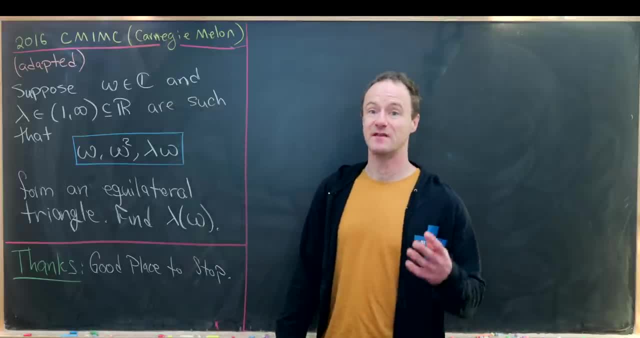 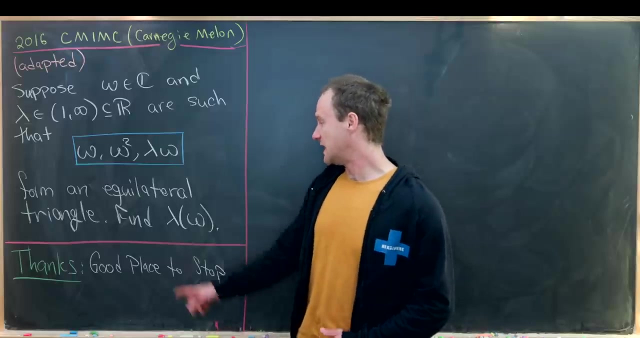 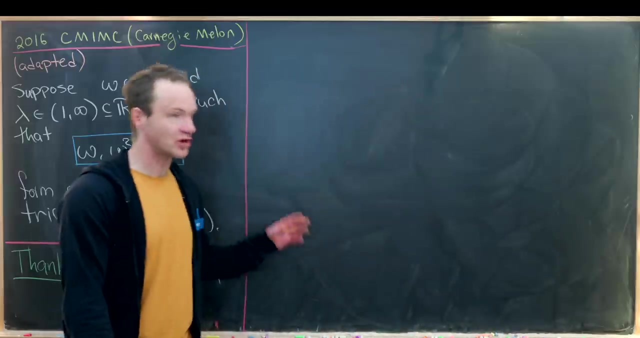 Furthermore, omega and lambda satisfy the following condition: Omega, omega squared, and lambda times omega form an equilateral triangle, And that equilateral triangle is living in the complex plane, And our goal is to find lambda as a function of omega. Okay, so let's maybe get a picture of this situation on the board. 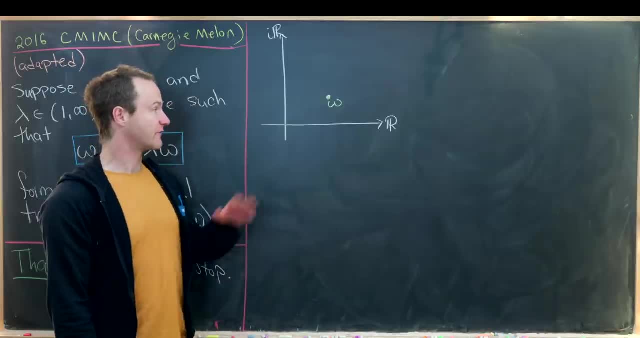 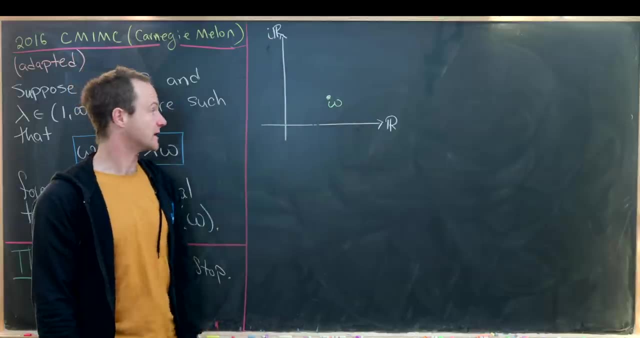 And then we'll go from there. So I've started our picture, I've got my complex plane. The real axis is running horizontally and the imaginary axis is running vertically. So I've put my complex number omega in the first quadrant. But this could be generalized to any quadrant. 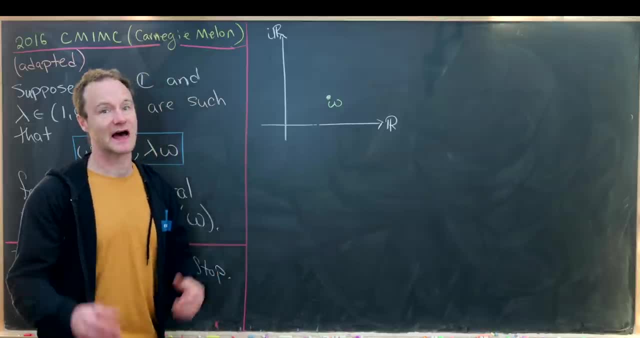 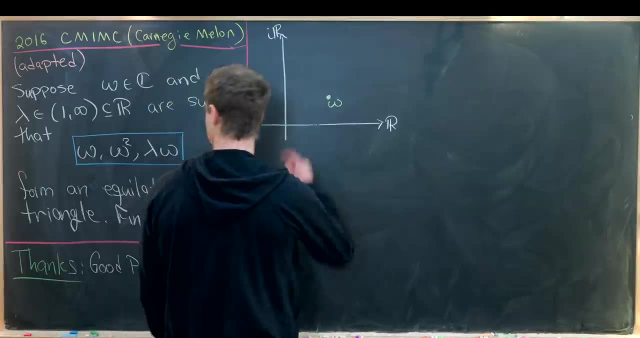 Remember. this is just to get us thinking. This is just to get us thinking about some, maybe like algebraic properties that are the relation between lambda and omega. Okay, so now that we've got omega, let's write down one of these other numbers in the complex plane. 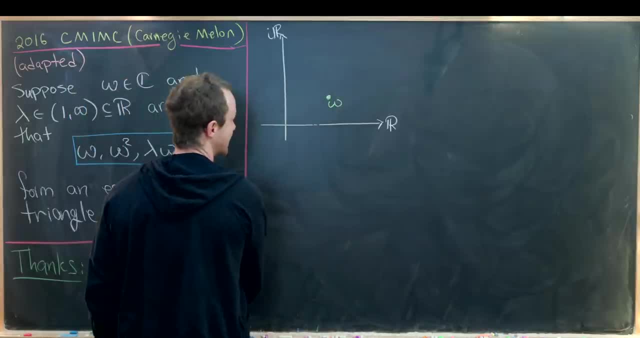 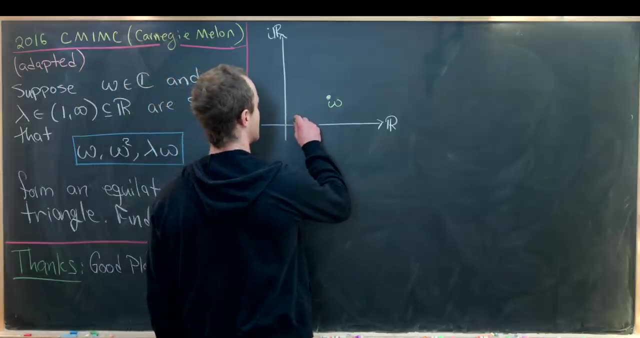 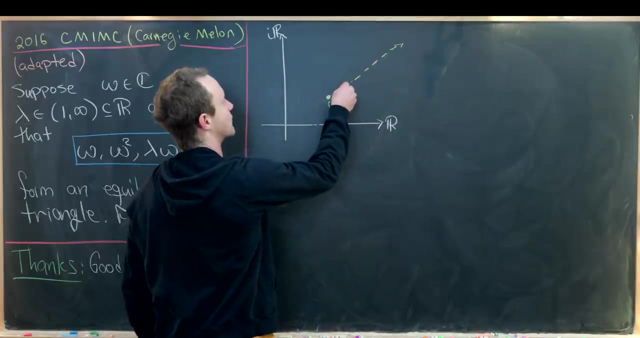 Maybe the easiest one to do will be lambda times omega. So since lambda is bigger than 1, we know that lambda times omega will be on the positive ray emanating from the origin going through omega. So there's my equation, So there's my ray from the origin going through omega. 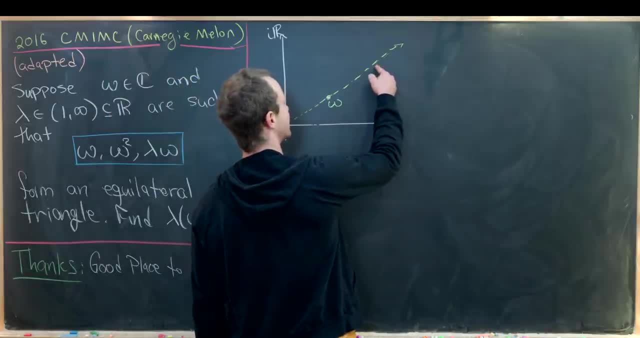 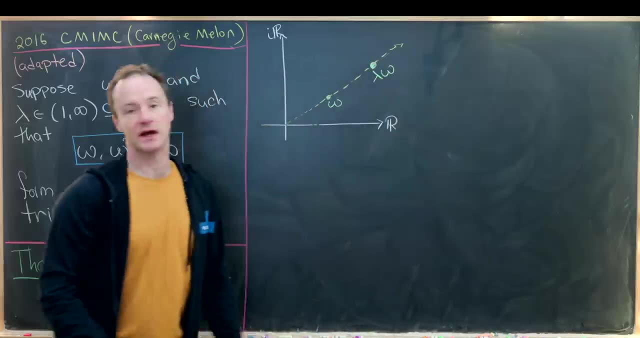 And again, because lambda is bigger than 1, we know it's going to be further out than omega. So I'll just put right here: this is lambda times omega, like that. Okay, so that's looking good. And then omega squared will be related to omega in that it will have a square of the distance from the origin. 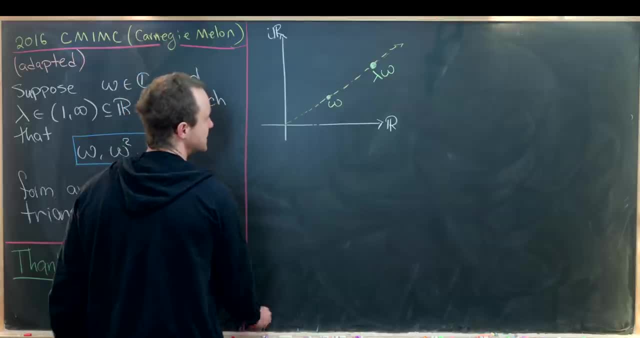 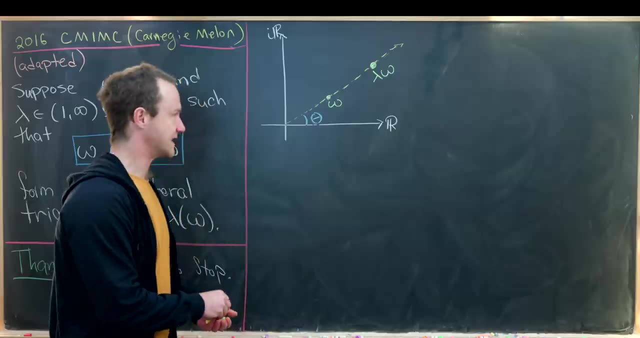 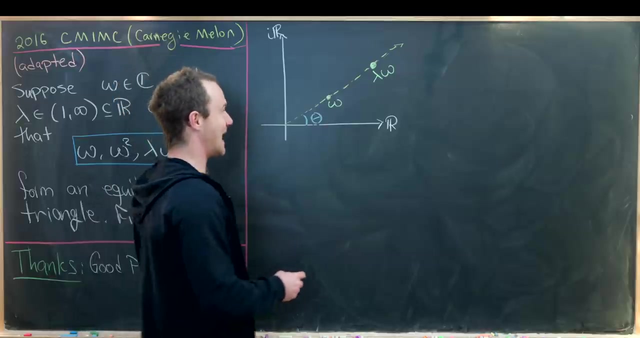 And the argument will be doubled. So here, If theta is the argument of omega, then 2 theta will be the argument of omega squared. But furthermore we know that this completes an equilateral triangle, So we can actually just like eyeball it and put omega squared. maybe right about here. 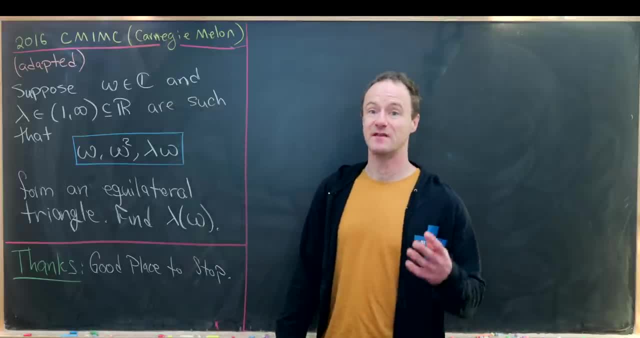 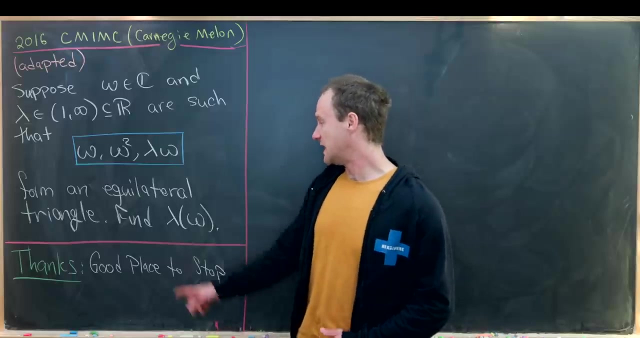 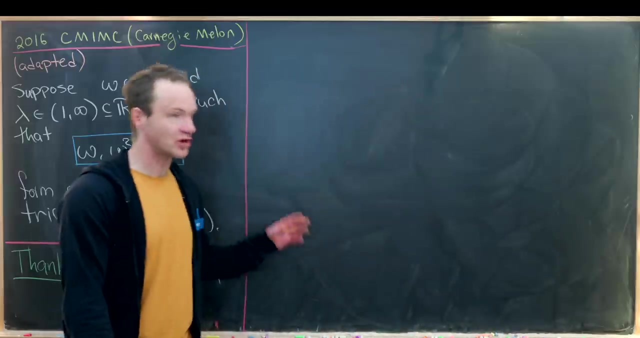 Furthermore, omega and lambda satisfy the following condition: Omega, omega squared, and lambda times omega form an equilateral triangle, And that equilateral triangle is living in the complex plane, And our goal is to find lambda as a function of omega. Okay, so let's maybe get a picture of this situation on the board. 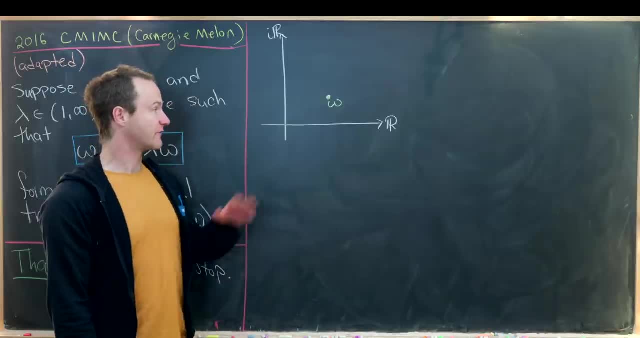 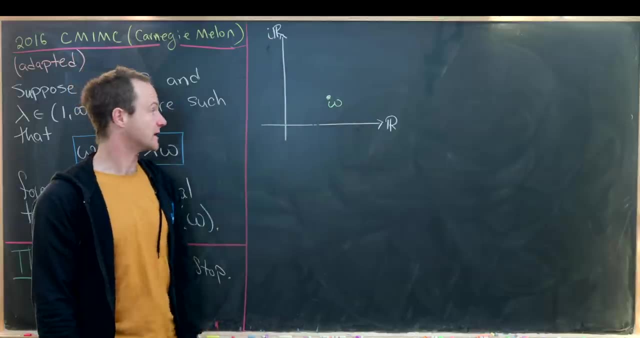 And then we'll go from there. So I've started our picture, I've got my complex plane. The real axis is running horizontally and the imaginary axis is running vertically. So I've put my complex number omega in the first quadrant. But this could be generalized to any quadrant. 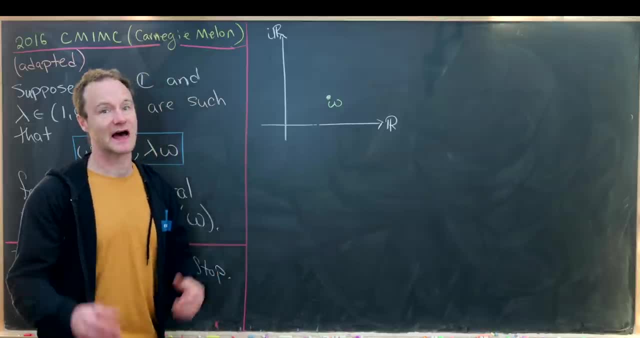 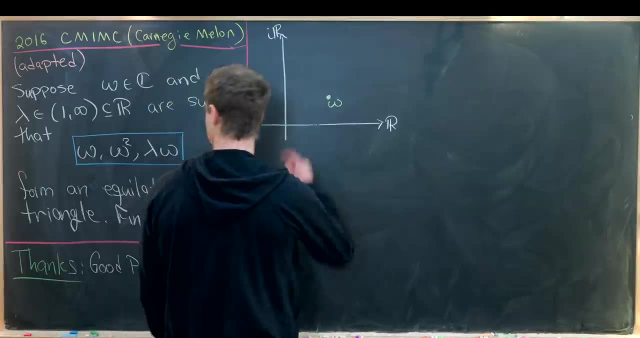 Remember. this is just to get us thinking. This is just to get us thinking about some, maybe like algebraic properties that are the relation between lambda and omega. Okay, so now that we've got omega, let's write down one of these other numbers in the complex plane. 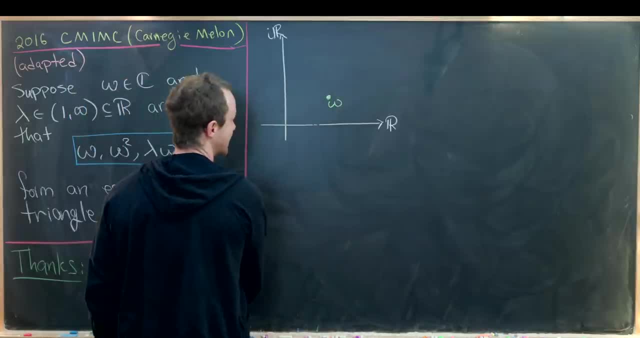 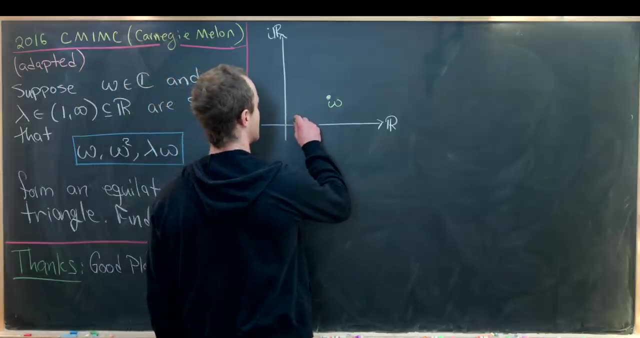 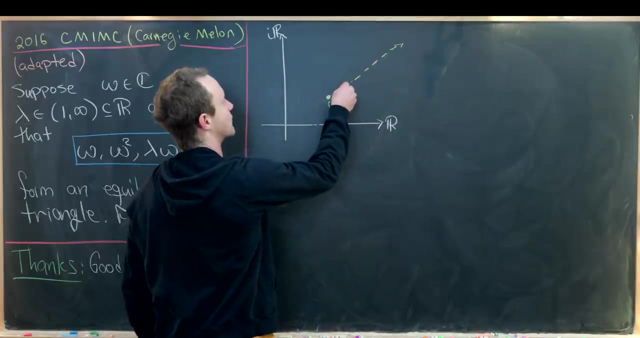 Maybe the easiest one to do will be lambda times omega. So since lambda is bigger than 1, we know that lambda times omega will be on the positive ray emanating from the origin going through omega. So there's my equation, So there's my ray from the origin going through omega. 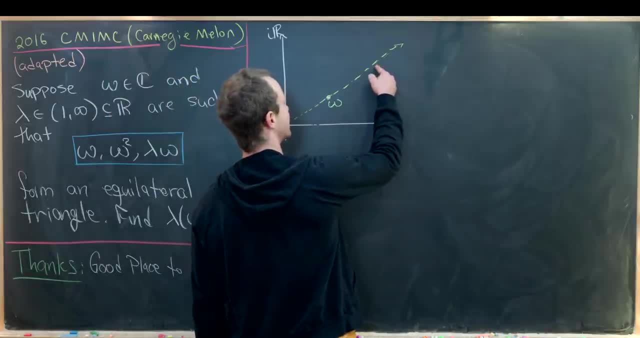 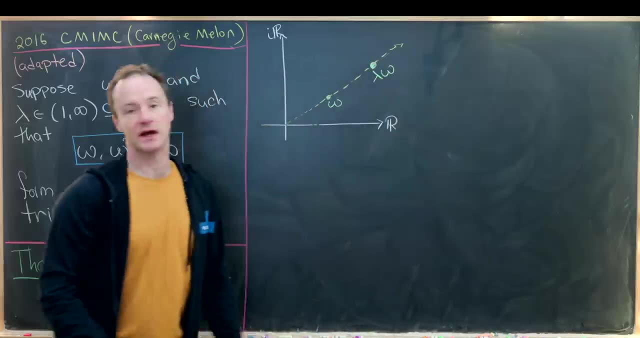 And again, because lambda is bigger than 1, we know it's going to be further out than omega. So I'll just put right here: this is lambda times omega, like that. Okay, so that's looking good. And then omega squared will be related to omega in that it will have a square of the distance from the origin. 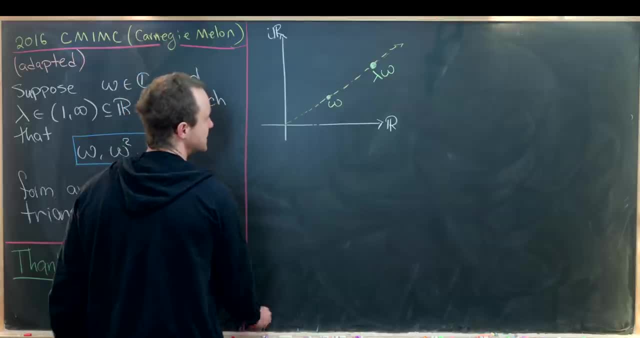 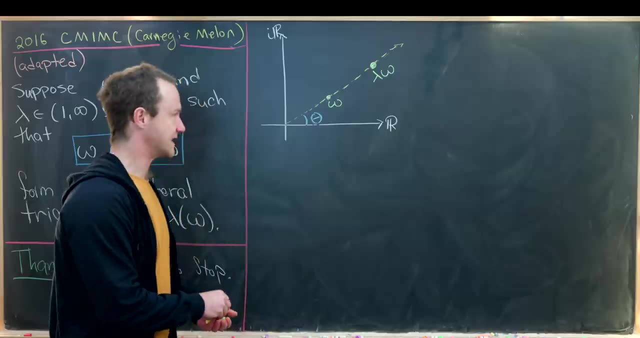 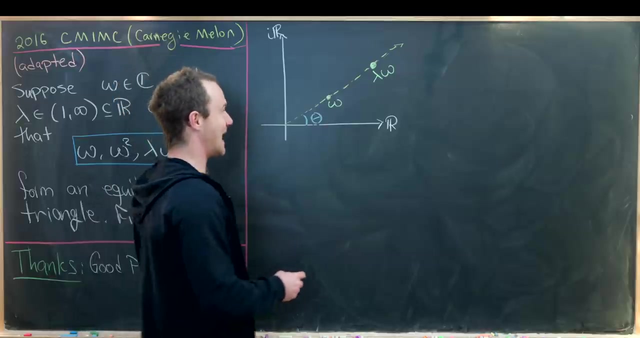 And the argument will be doubled. So here, If theta is the argument of omega, then 2 theta will be the argument of omega squared. But furthermore we know that this completes an equilateral triangle, So we can actually just like eyeball it and put omega squared. maybe right about here. 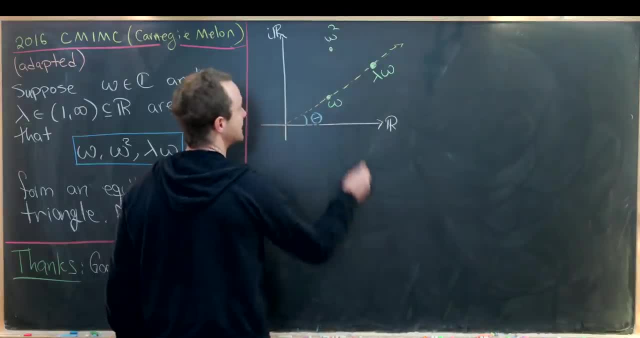 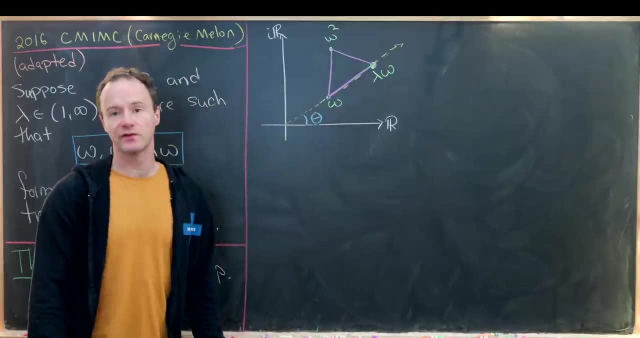 So here's omega squared, And we did that in a way so that we have something that looks pretty much like an equilateral triangle. Okay, so that's looking good, And now we're going to use a well-known fact, And that is: multiplication by a complex number is a similarity on the complex plane. 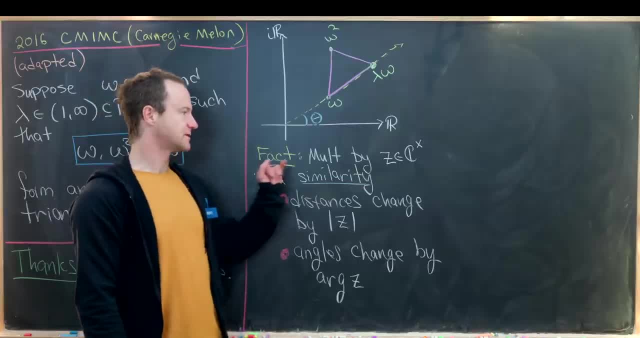 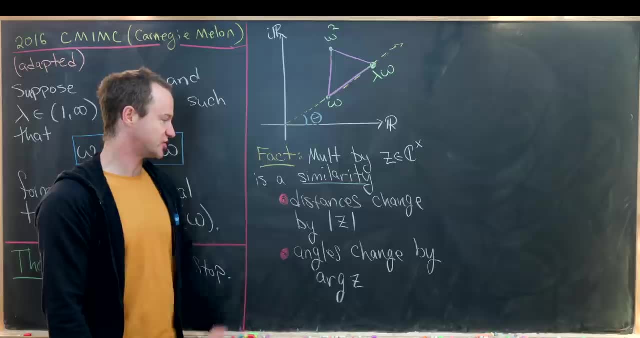 So let's get that fact on the board. So, like I just said, multiplying by a non-zero complex number is a similarity of the complex plane. In particular, the distances change by the modulus of z And the angles change by the argument of z. 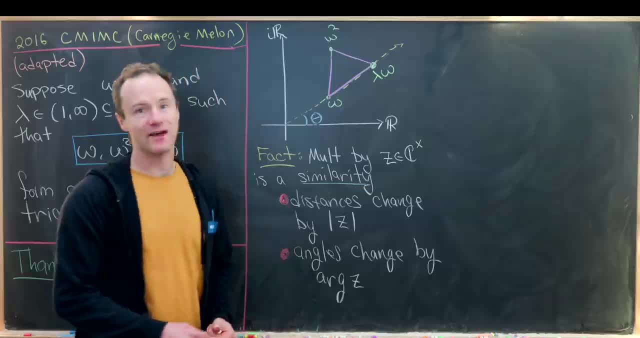 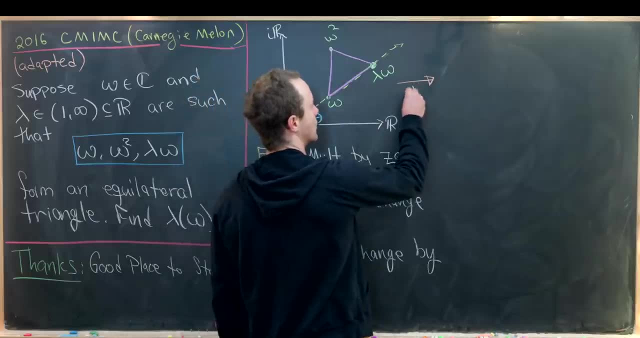 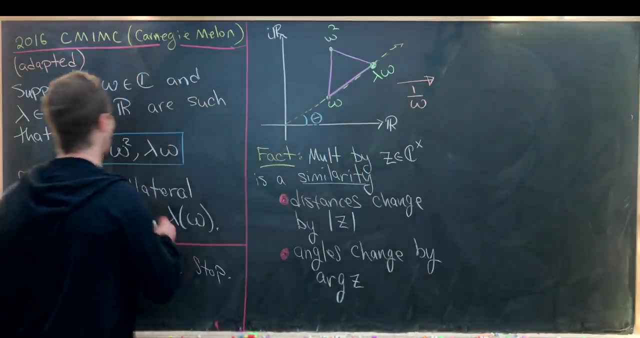 So, looking at our picture, There's probably an advantageous complex number to multiply by And that advantageous complex number will be 1 over omega. And I guess I should have pointed out at the beginning that omega is not equal to 0. So we'll just add that in by saying that omega is in the non-zero set of the complex numbers. 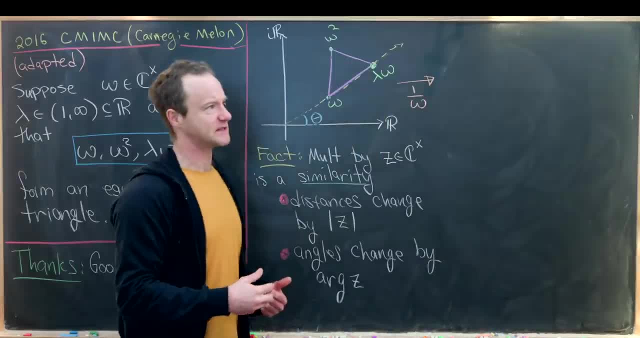 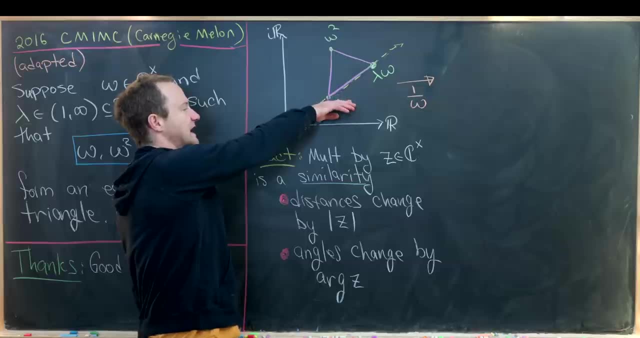 If we put a little x here, that's what that means. That's because it forms a multiplicative group. So let's see what multiplying by 1 over omega looks like. So it'll rotate everything by negative theta. That's because it's 1 over omega. 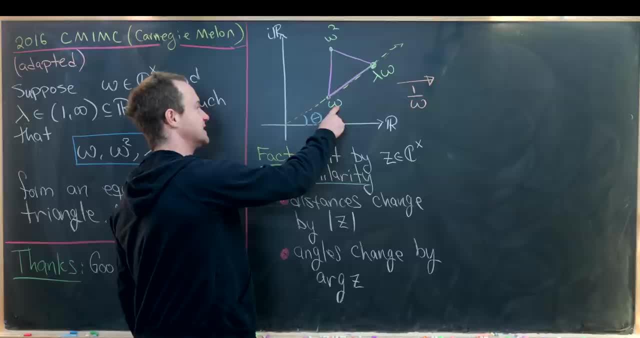 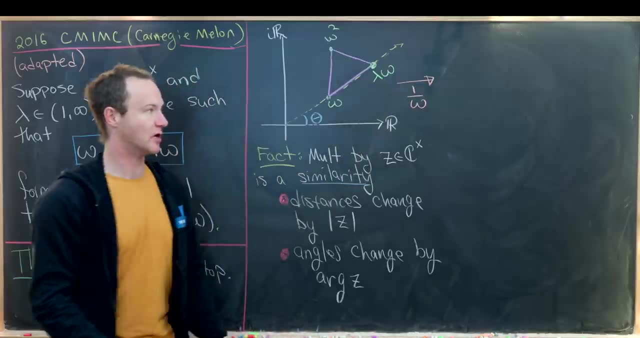 And then it'll scale everything by omega. So this will go to the point 1 on the real axis, This will go to the point lambda on the real axis, And then omega squared will become omega Okay. so let's draw that picture over there. 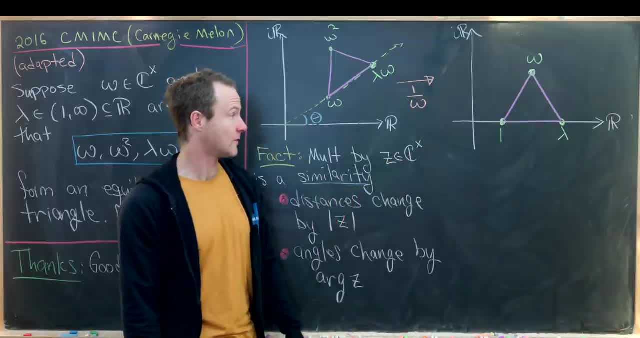 Okay, so we end up with the following triangle, which is nice now because it lives on this real axis. And since it lives on this real axis, we're going to talk about the measurement of these sides pretty easily. So notice: the distance from 1 to lambda will be lambda minus 1.. 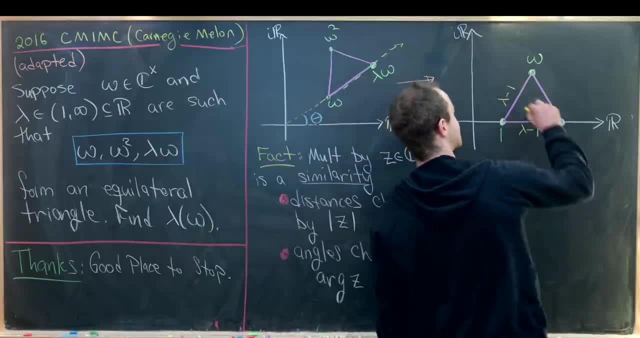 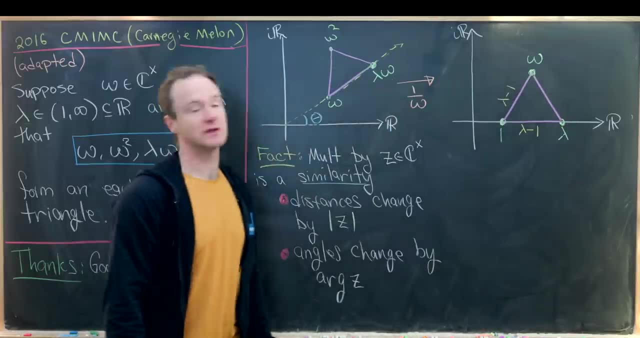 And then, since this is an equilateral triangle, all of these distances will also be lambda minus 1.. So I'll just put one more in there. But this one right here is also lambda minus 1,, or has length, lambda minus 1.. 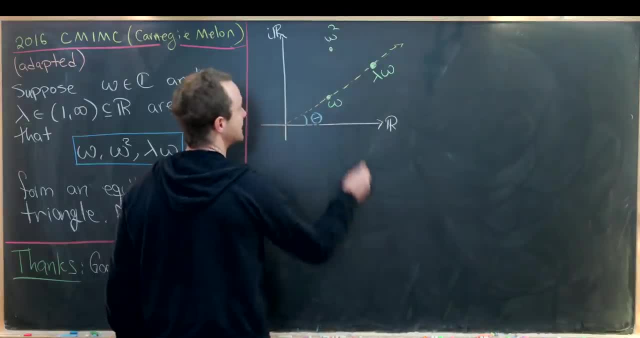 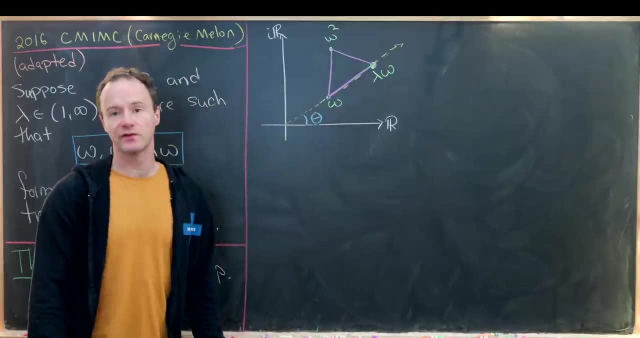 So here's omega squared, And we did that in a way so that we have something that looks pretty much like an equilateral triangle. Okay, so that's looking good, And now we're going to use a well-known fact, And that is: multiplication by a complex number is a similarity on the complex plane. 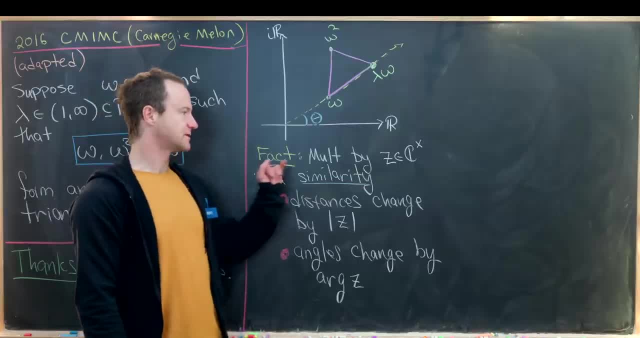 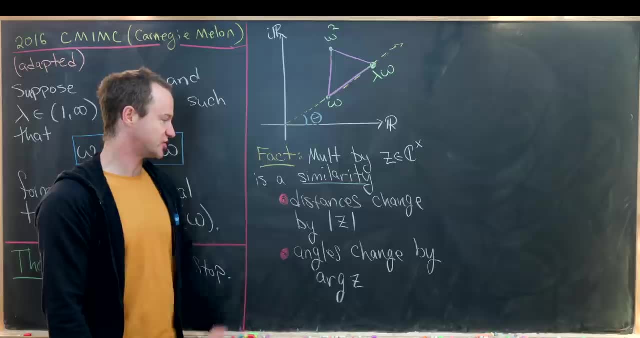 So let's get that fact on the board. So, like I just said, multiplying by a non-zero complex number is a similarity of the complex plane. In particular, the distances change by the modulus of z And the angles change by the argument of z. 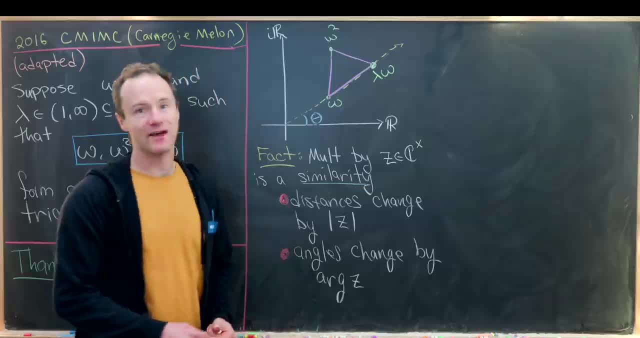 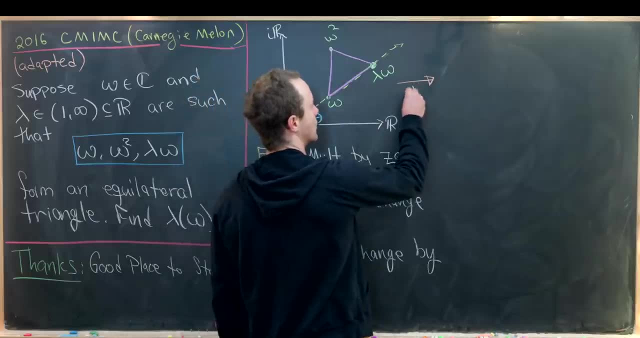 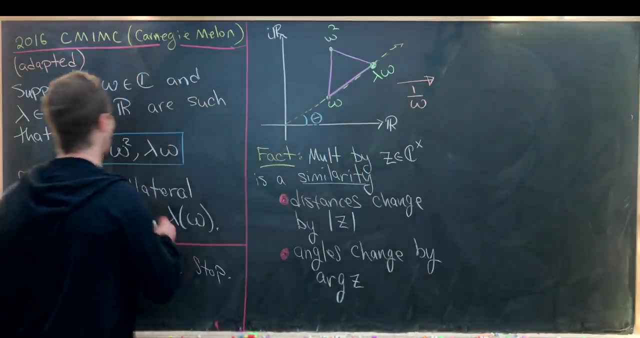 So, looking at our picture, There's probably an advantageous complex number to multiply by And that advantageous complex number will be 1 over omega. And I guess I should have pointed out at the beginning that omega is not equal to 0. So we'll just add that in by saying that omega is in the non-zero set of the complex numbers. 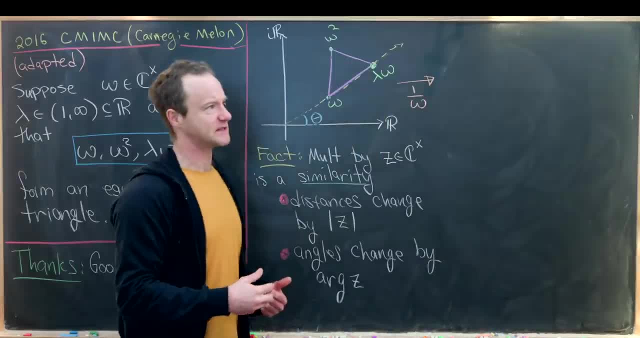 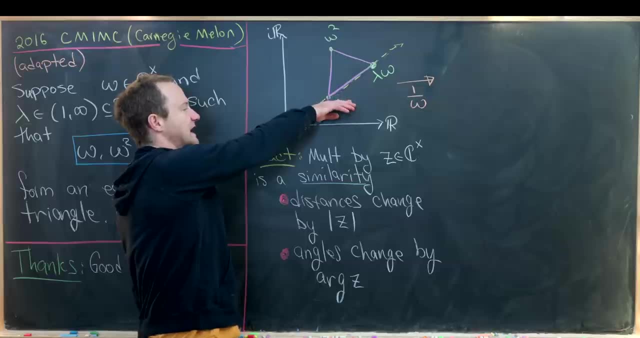 If we put a little x here, that's what that means. That's because it forms a multiplicative group. So let's see what multiplying by 1 over omega looks like. So it'll rotate everything by negative theta. That's because it's 1 over omega. 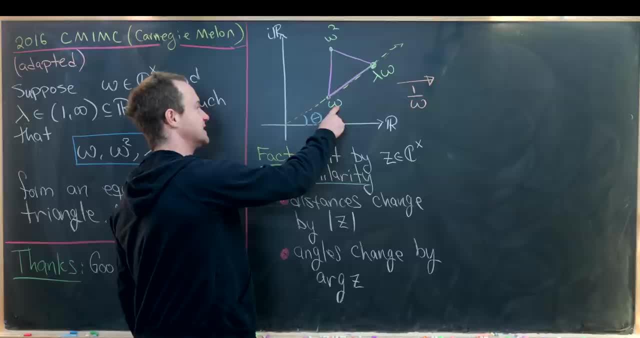 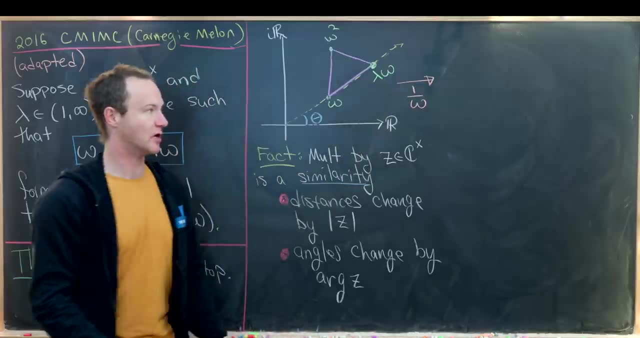 And then it'll scale everything by omega. So this will go to the point 1 on the real axis, This will go to the point lambda on the real axis, And then omega squared will become omega Okay. so let's draw that picture over there. 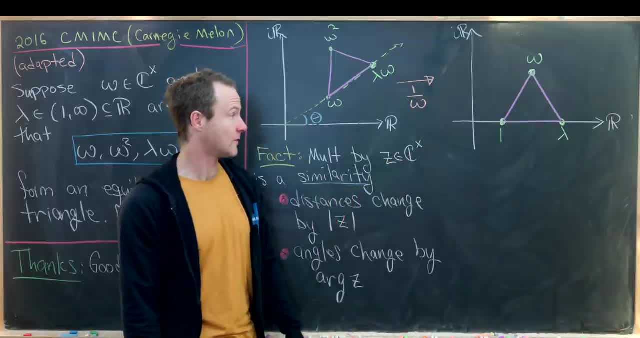 Okay, so we end up with the following triangle, which is nice now because it lives on this real axis. And since it lives on this real axis, we're going to talk about the measurement of these sides pretty easily. So notice: the distance from 1 to lambda will be lambda minus 1.. 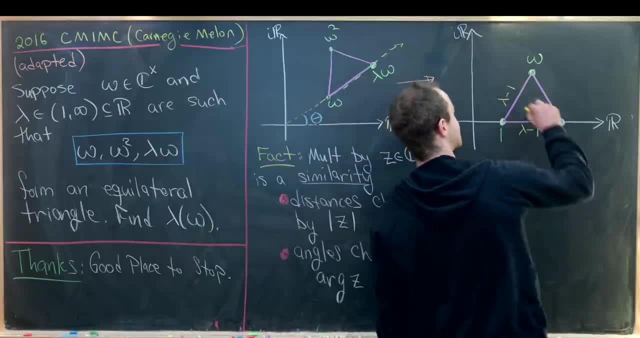 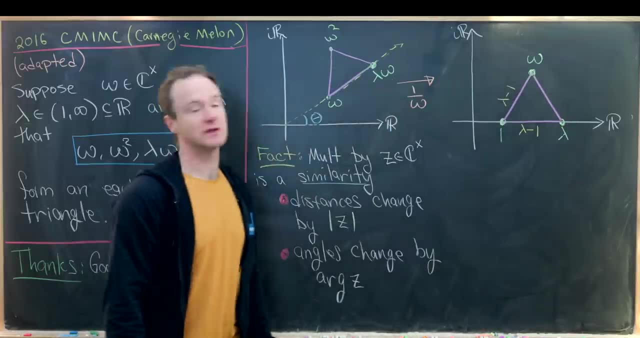 And then, since this is an equilateral triangle, all of these distances will also be lambda minus 1.. So I'll just put one more in there. But this one right here is also lambda minus 1,, or has length, lambda minus 1.. 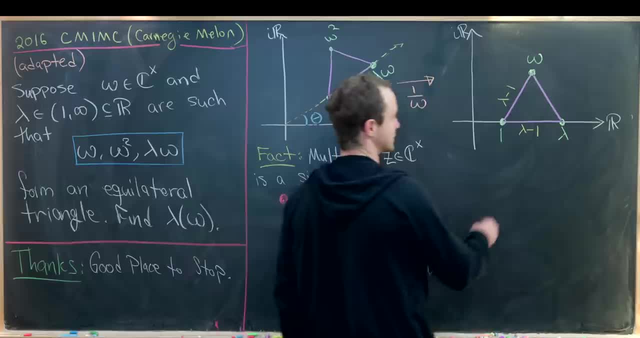 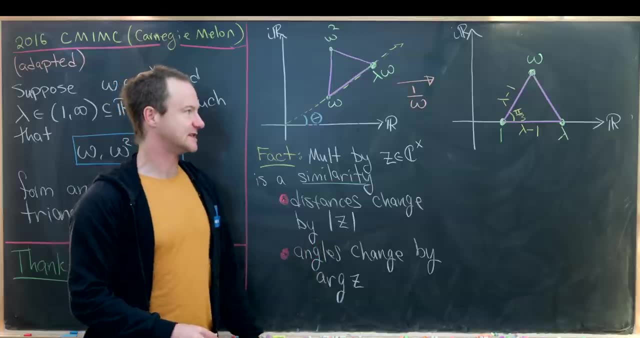 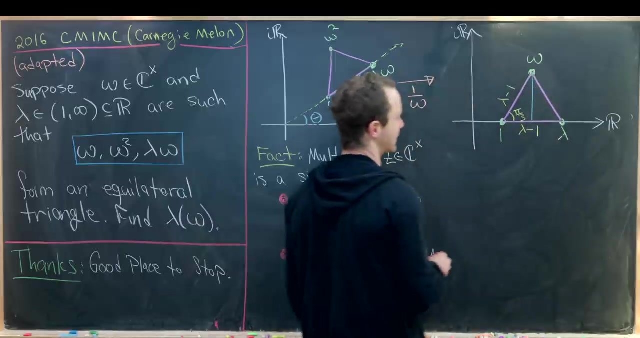 Furthermore, we know the angle measure of all of these angles as well. So this angle will be pi over 3, or 60 degrees Again, because that's an equilateral triangle. And now let's let that fill in the height of this triangle, which we can calculate with trigonometry. 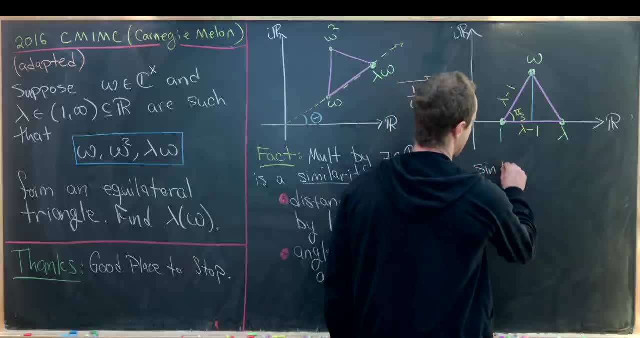 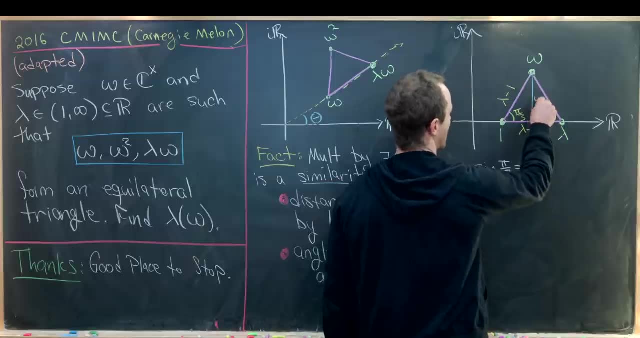 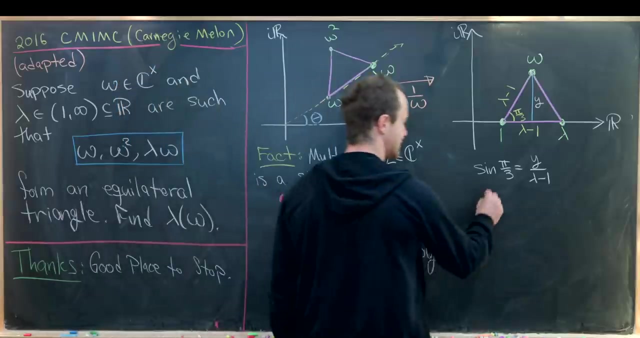 So let's notice that we know that sine of pi over 3 will be equal to this height, which I'll maybe call y. So let's put a y in here, over the hypotenuse, which is lambda minus 1.. Furthermore, we know sine of pi over 3 is the square root of 3 over 2.. 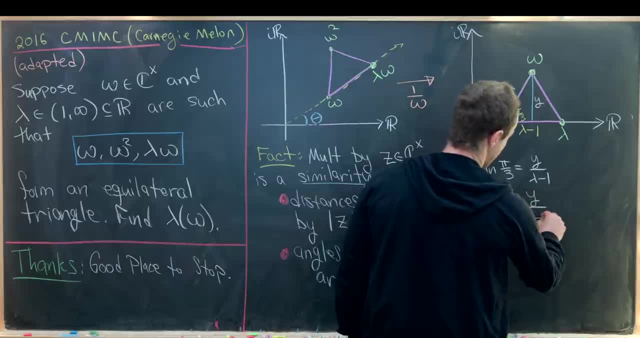 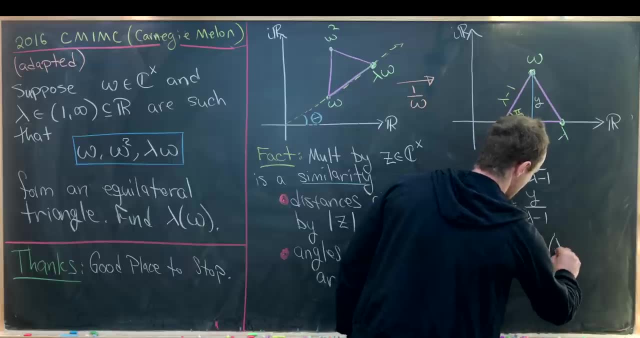 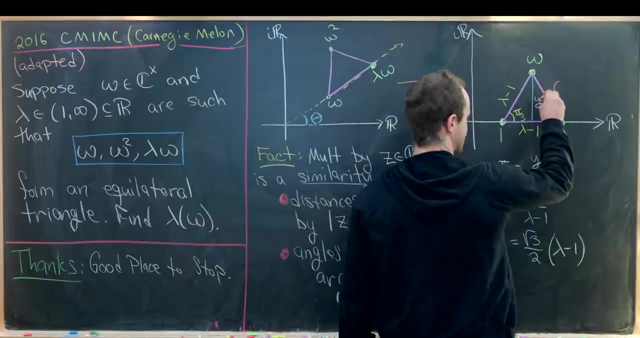 Okay, So that's equal to y over lambda minus 1, telling us that y is equal to the square root of 3 over 2 times the quantity lambda minus 1.. So we can maybe add that in here. So maybe I'll just do it like this. 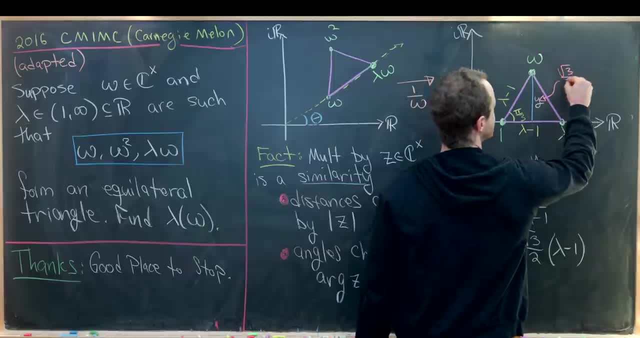 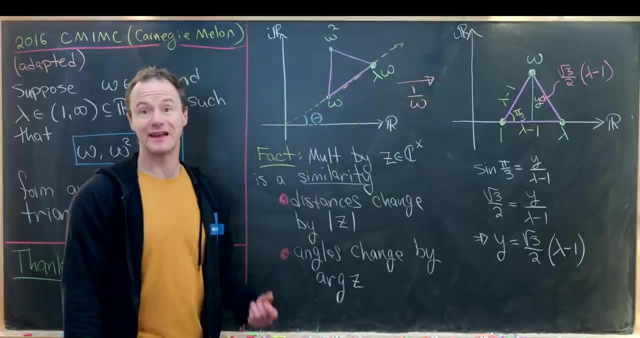 This is equal to the square root of 3 over 2 times lambda minus 1.. And now that we've got that measurement made, we're actually ready to finish this thing off, But we need a little bit more room. So this is the picture that we ended up with on the last board. 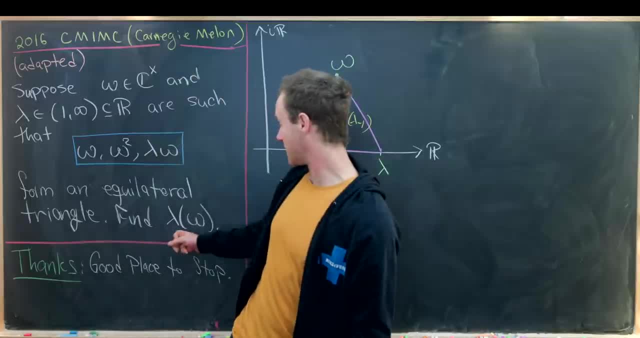 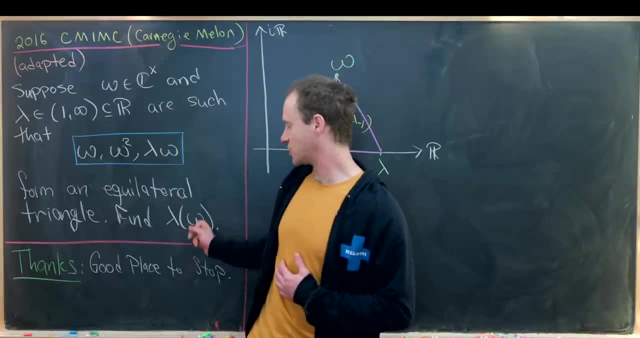 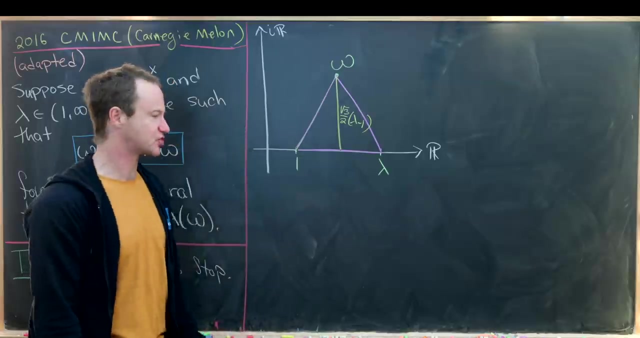 And now we have enough information to write a lambda as a function of omega. And in fact, not only will lambda be a function of omega, but it will be a function of the modulus of omega, or the distance of omega from the origin, which is maybe a little bit stronger of a condition. 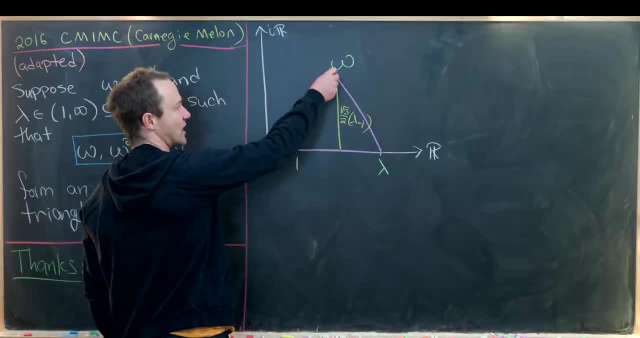 So, in order to see that we need to introduce another triangle into this situation, So the triangle will be in this piece. It's a peach color, So I'll draw it like this. So notice, the hypotenuse has distance omega or measure omega. 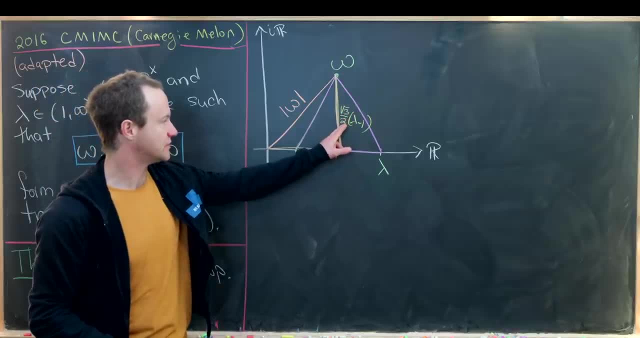 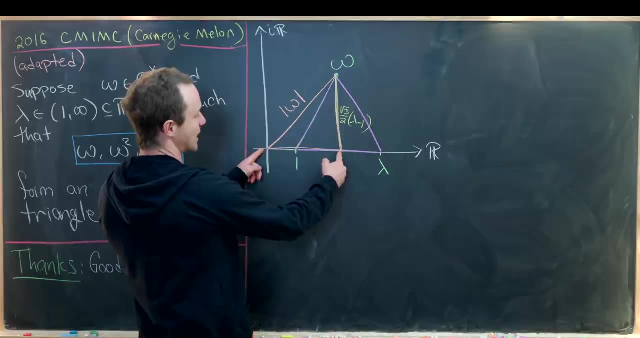 And then here this height is the square root of 3 over 2 times lambda minus 1.. And then we can figure out this distance as well, which is not too hard, And then this point right here will be the average of lambda n1.. 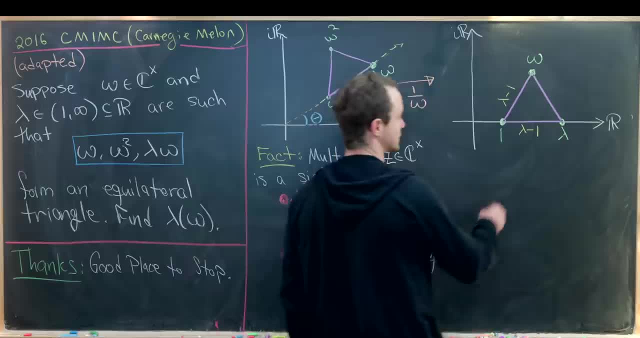 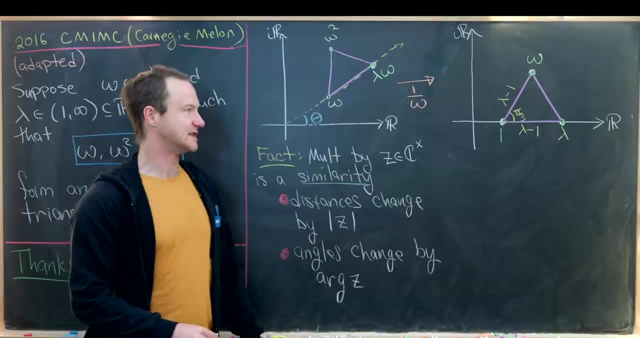 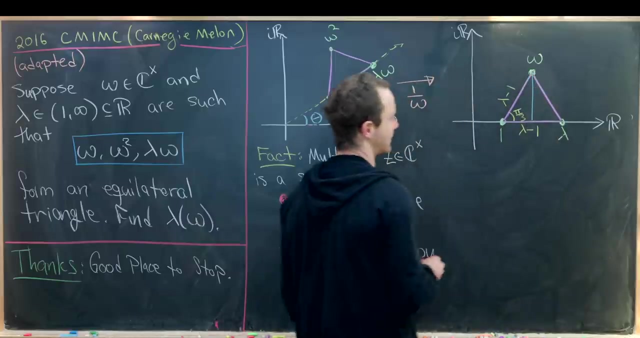 Furthermore, we know the angle measure of all of these angles as well. So this angle will be pi over 3, or 60 degrees Again, because that's an equilateral triangle. And now let's let that fill in the height of this triangle, which we can calculate with trigonometry. 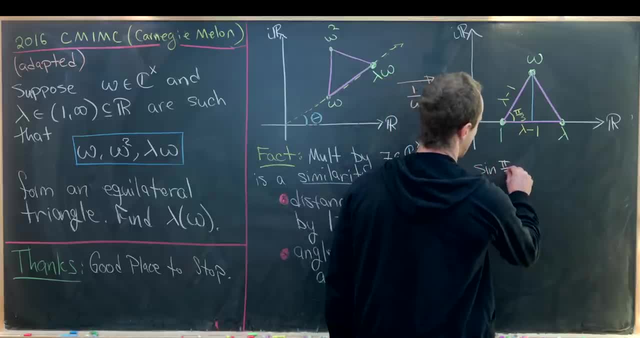 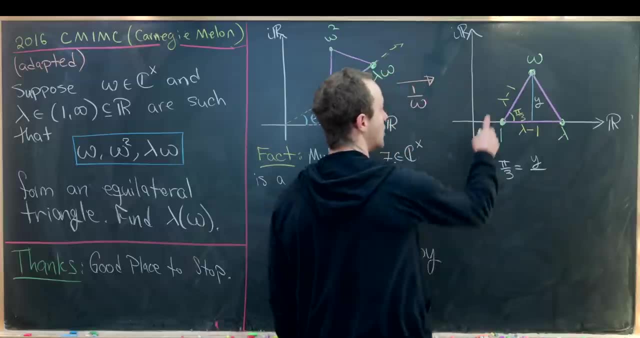 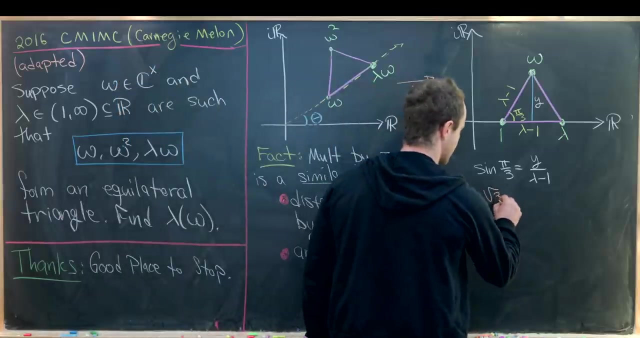 So let's notice that we know that sine of pi over 3 will be equal to this height, which I'll maybe call y. So let's put a y in here, over the hypotenuse, which is lambda minus 1.. Furthermore, we know sine of pi over 3 is the square root of 3 over 2.. 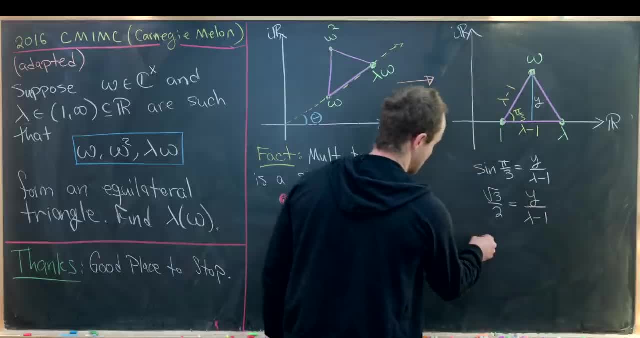 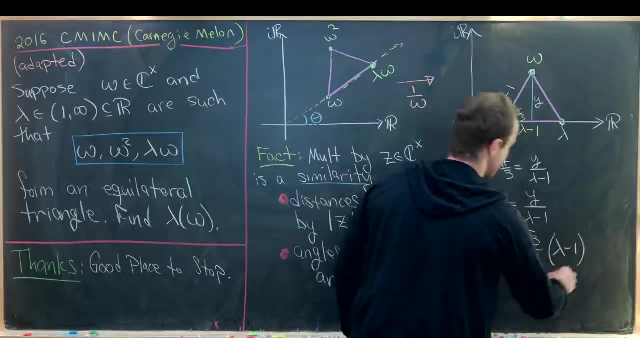 So that's equal to y over lambda minus 1, telling us that y is equal to the square root of 3 over 2 times the quantity lambda minus 1.. So we can maybe add that in here. So maybe I'll just do it like this: 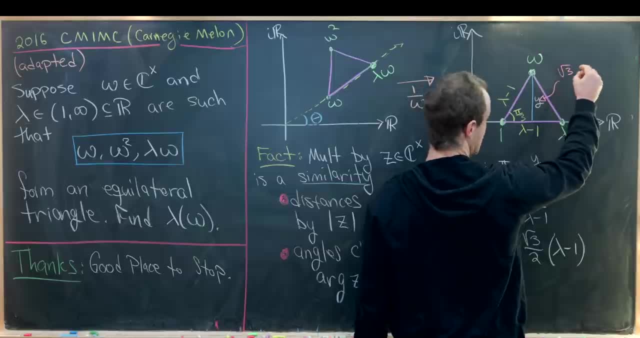 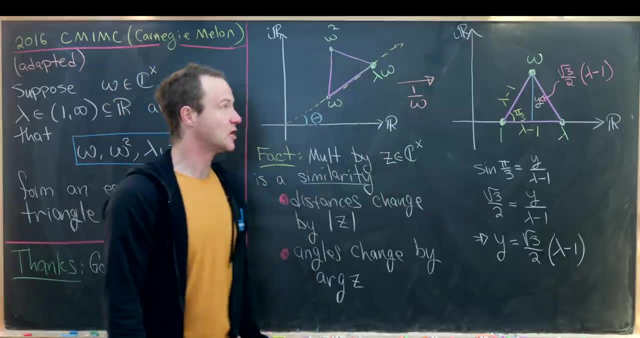 This is equal to the square root of 3 over 2 times lambda minus 1.. And now that we've got that measurement made, we're actually ready to finish this thing off, But we need a little bit more room. So this is the picture that we ended up with on the last board. 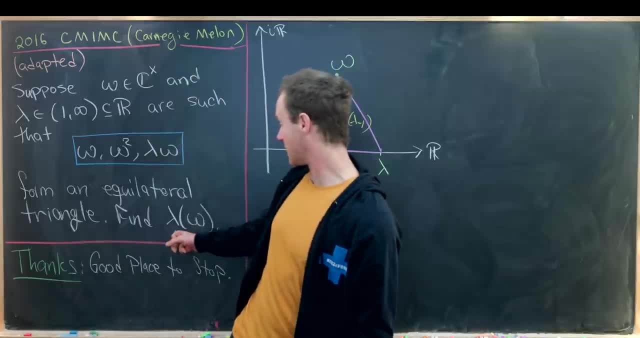 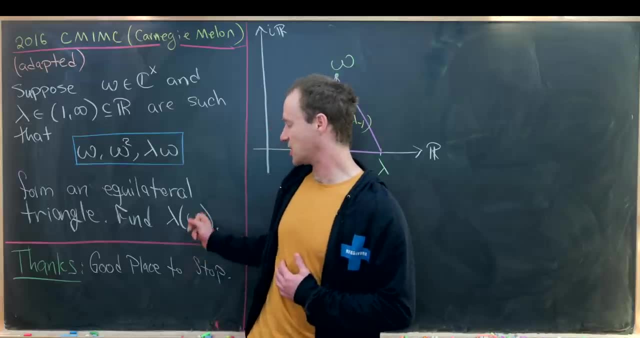 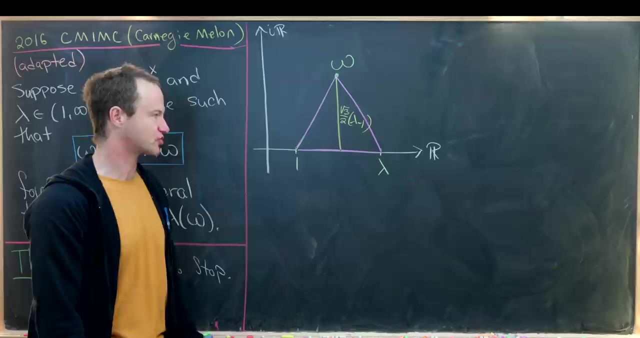 And now we have enough information to write lambda as a function of omega. And, in fact, not only will lambda be a function of omega, but it will be a function of the modulus of omega, or the distance of omega from the origin, which is maybe a little bit stronger of a condition. 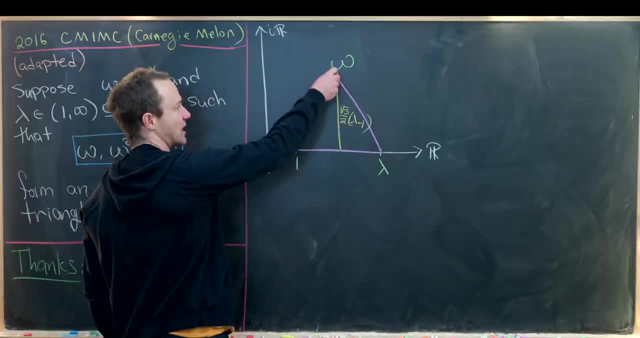 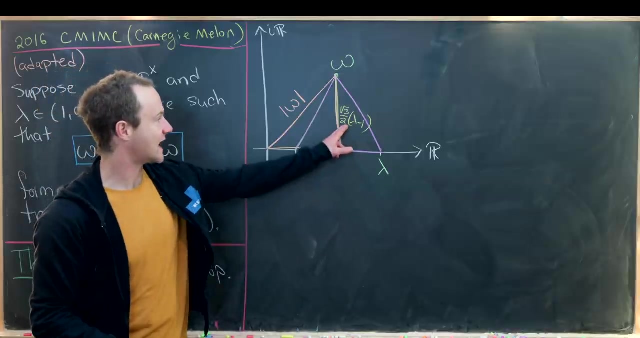 So, in order to see that we need to introduce another triangle into this situation, So the triangle will be in this peach color, So I'll draw it like this. So notice, the hypotenuse has distance omega or measure omega. And then here this height is the square root of 3 over 2 times lambda minus 1.. 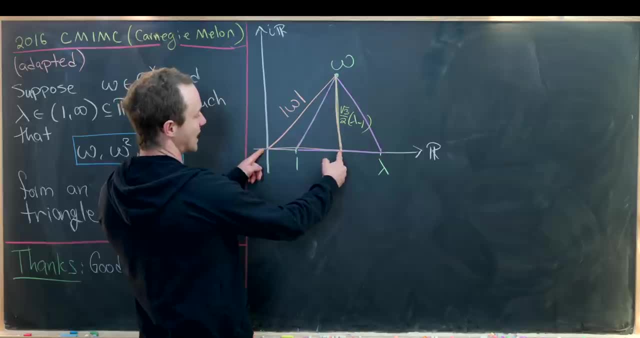 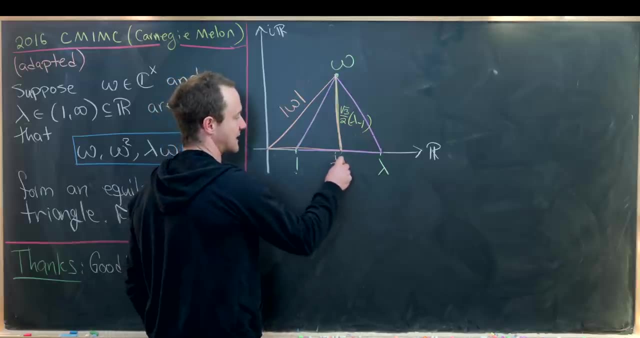 And then we can figure out this distance as well, which is not too hard. And then this point right here will be the average of lambda n1.. So that'll be lambda plus 1 over 2.. Now we've got a nice setup. 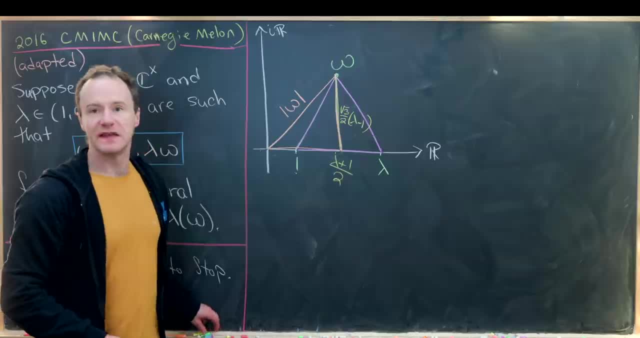 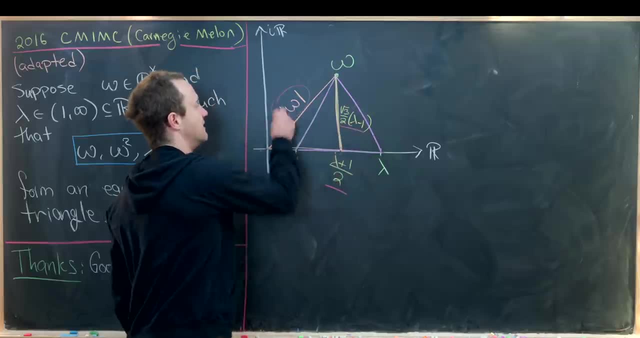 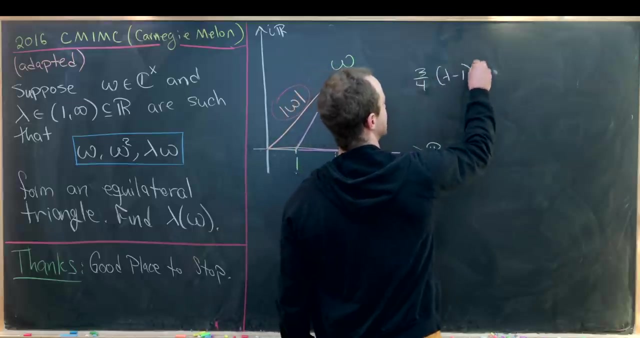 So that'll be lambda plus 1 over 2.. Now we've got a nice setup where we can apply the Pythagorean theorem to the triangle with these two side lengths and this guy as the length of the hypotenuse. So that's going to give us 3 over 4 times lambda minus 1 squared plus 1 over 4 times lambda plus 1 squared. 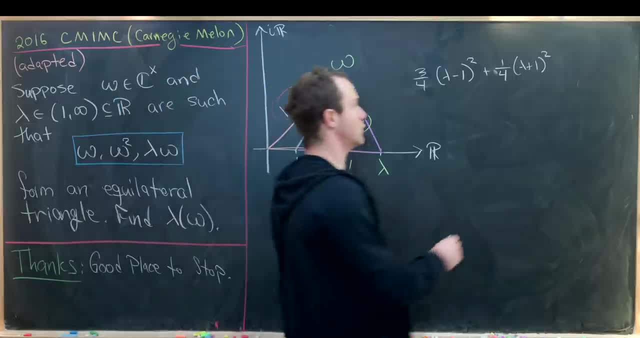 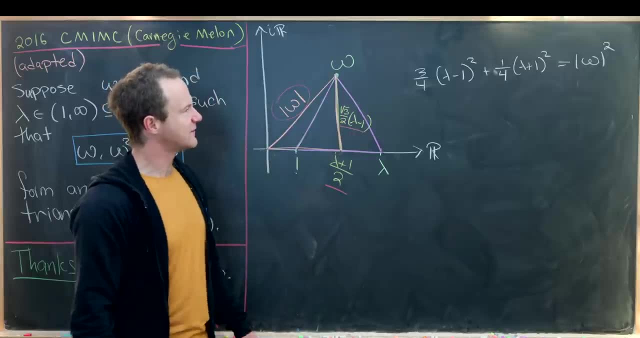 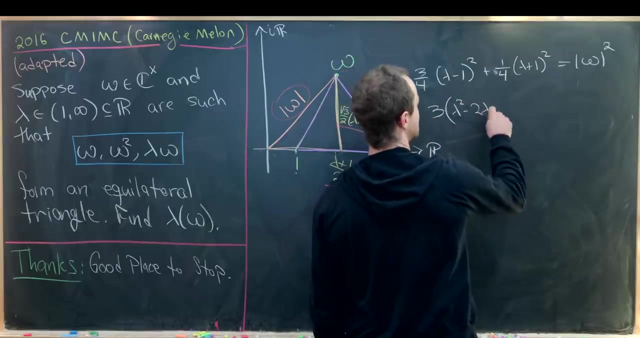 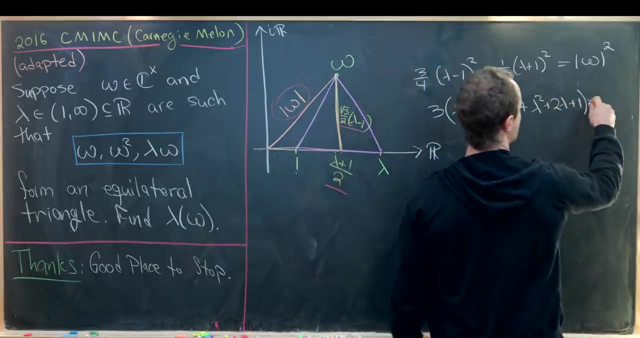 So that's from squaring these two side lengths equals the magnitude or the modulus of omega squared. Okay, great. So now let's see if we can simplify this a little bit. This will give us 3 times lambda squared minus 2. lambda plus 1 plus lambda squared plus 2 lambda plus 1 equals 4 times the magnitude of omega squared. 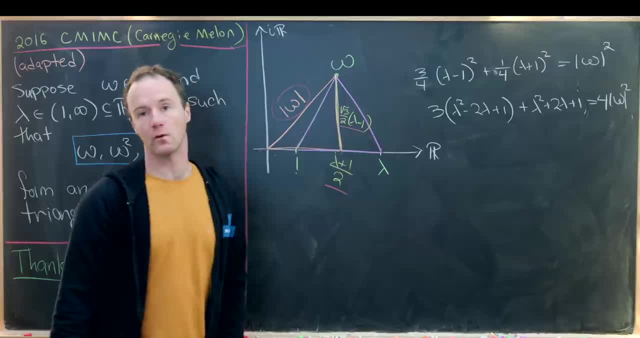 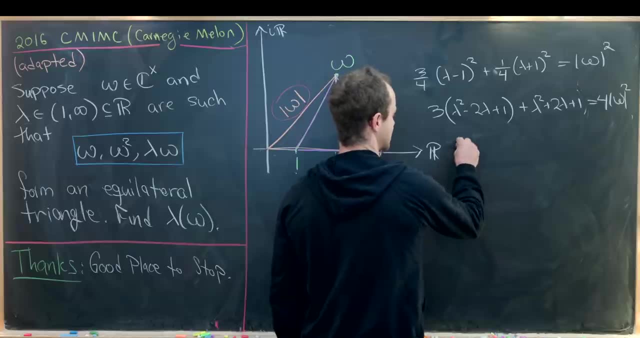 So I got that just by multiplying both sides of this equation by 4.. Okay, so now let's see if we can simplify a little bit. So I have 3 times lambda squared, 3 times lambda squared plus lambda squared, That gives me 4 lambda squared. 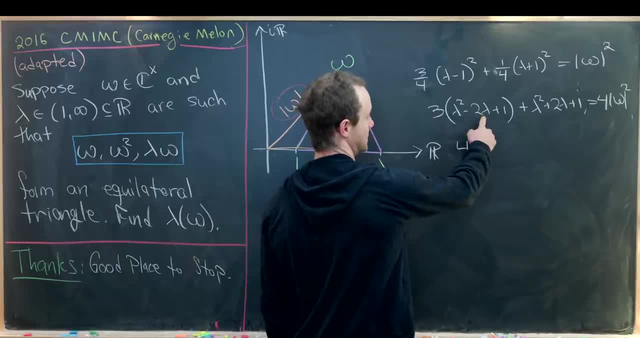 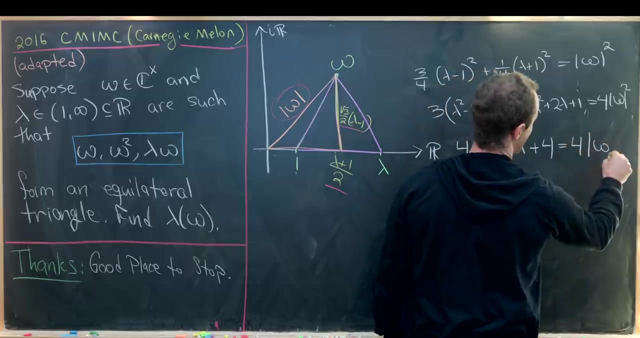 Then I'll have minus 6 lambda plus 2 lambda, So that's going to be minus 4 lambda. And then I have 3 times 1 plus 1. So that'll be plus 4.. Again, that equals 4 times the magnitude of omega squared. 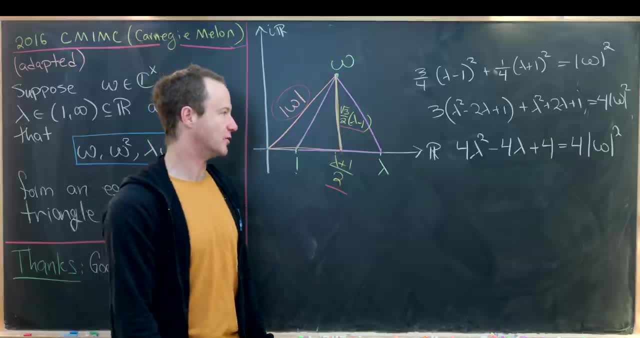 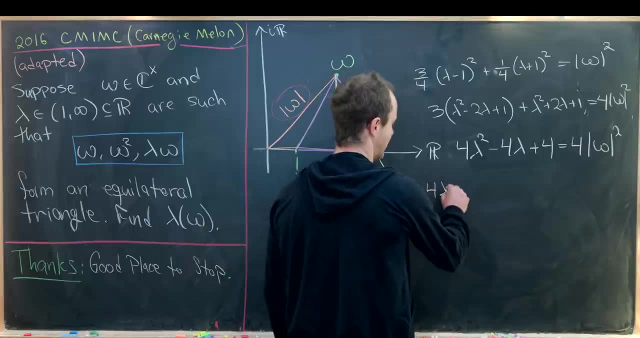 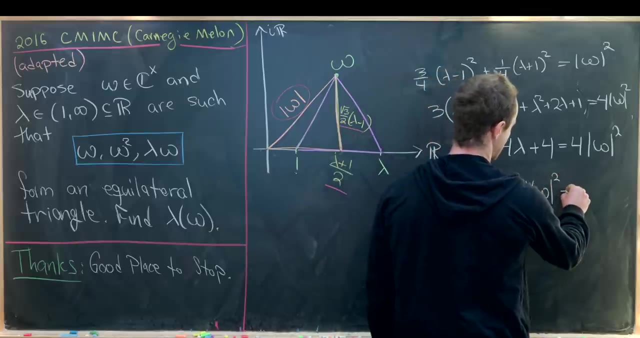 And now we can see here that we have almost a perfect square binomial. If we subtract 3 from both sides, we will have a perfect square binomial. So let's do that. We'll have 4 lambda squared minus 4. lambda plus 1 equals 4 times the modulus of omega squared minus 3.. 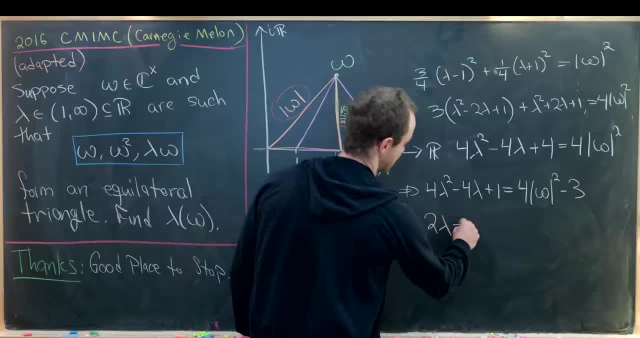 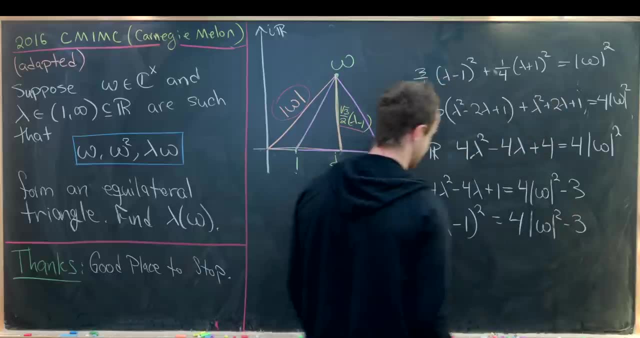 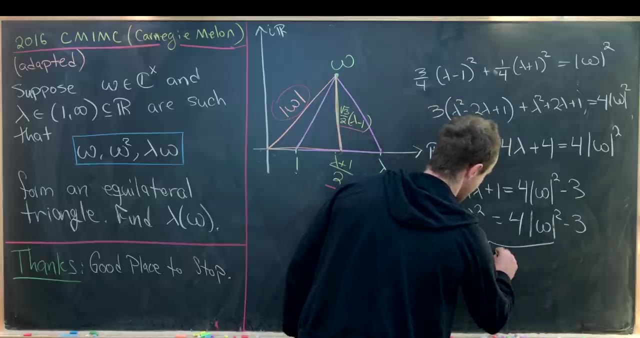 Then this factors like: 2 lambda minus 1, quantity squared equals 4 times omega squared minus 3.. We can take the square root of both sides We have: 2 lambda minus 1 equals the square root of 4 times omega squared minus 3.. 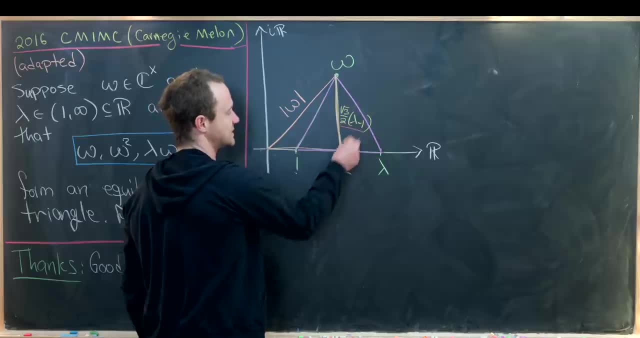 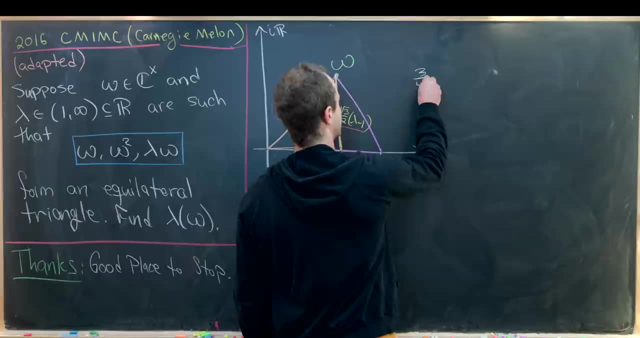 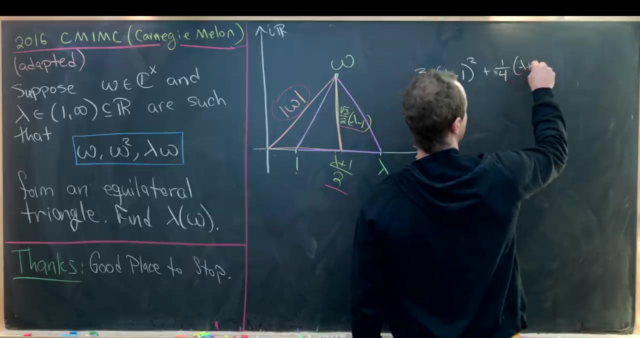 We can apply the Pythagorean theorem to the triangle with these two side lengths and this guy as the length of the hypotenuse. So that's going to give us 3 over 4 times lambda minus 1 squared, plus 1 over 4 times lambda plus 1 squared. 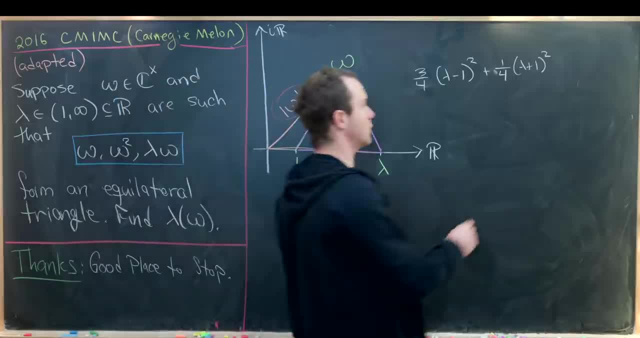 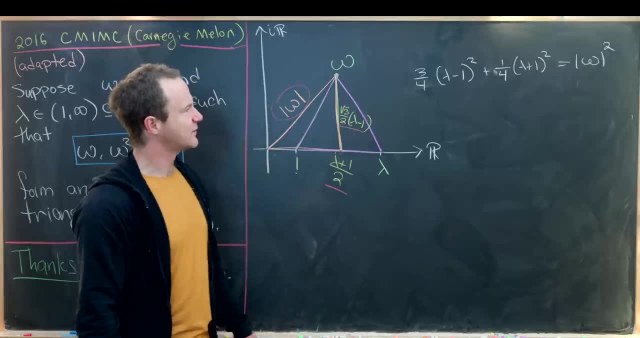 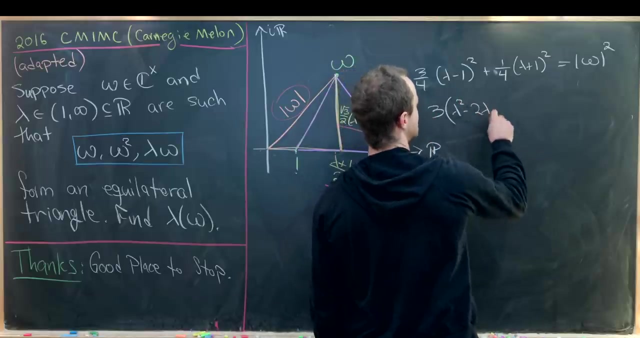 So that's from squaring these two side lengths equals the magnitude or the modulus of omega squared. Okay, great. So now let's see if we can simplify this. This will give us 3 times lambda squared minus 2 lambda plus 1. 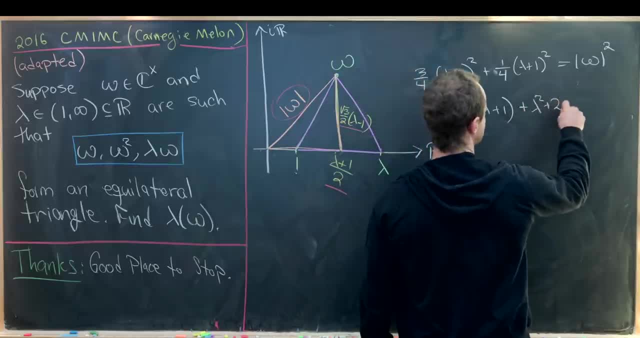 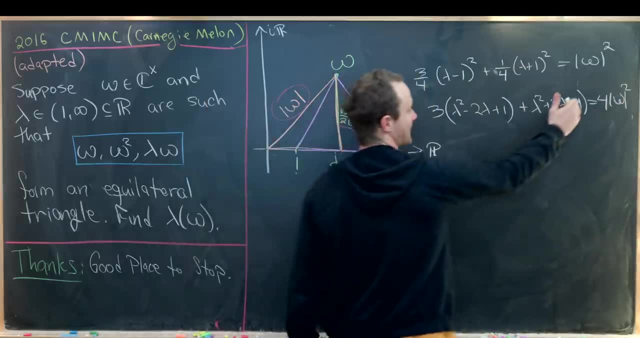 plus lambda squared plus 2. lambda plus 1 equals 4 times the magnitude of omega squared. So I got that just by multiplying both sides of this equation by 4.. Okay, so now let's see if we can simplify a little bit. 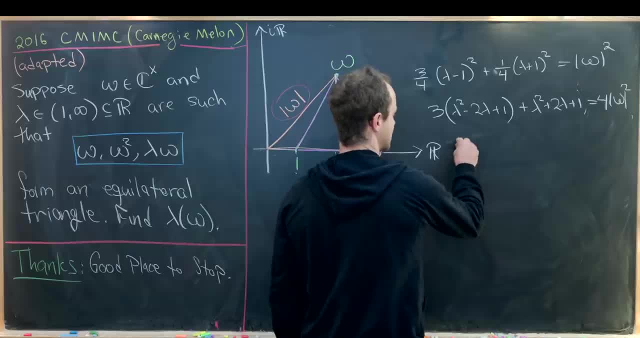 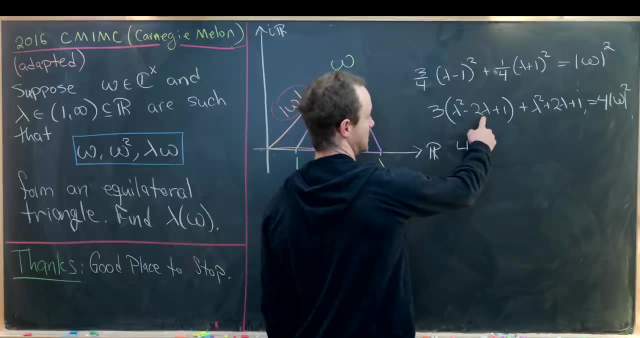 So I have 3 times lambda squared plus lambda squared. That gives me 4 lambda squared. Then I'll have minus 6 lambda plus 2 lambda. So that's going to be minus 4 lambda. And then I have 3 times 1 plus 1.. 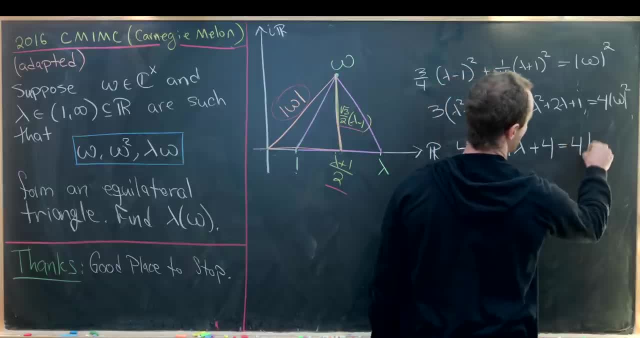 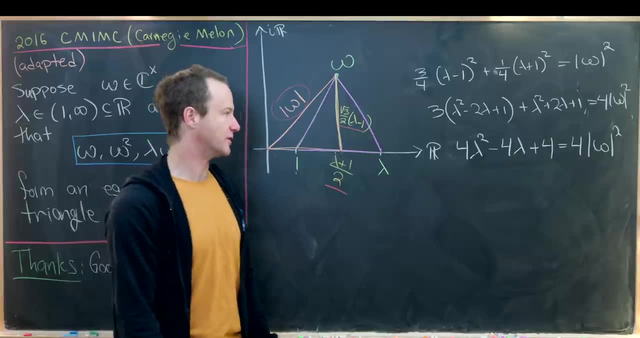 So that'll be plus 4.. Again, that equals 4 times the magnitude of omega squared. And now we can see here that we have almost a perfect square binomial. If we subtract 3 from both sides, we will have a perfect square binomial. 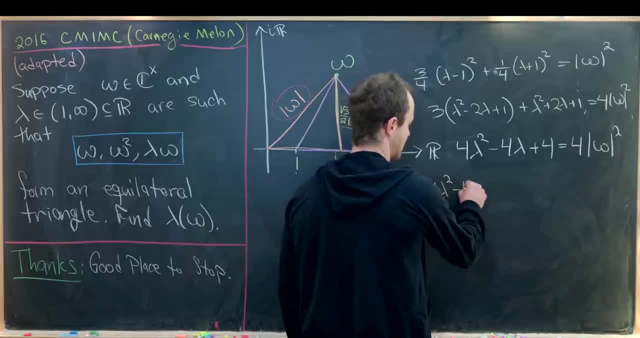 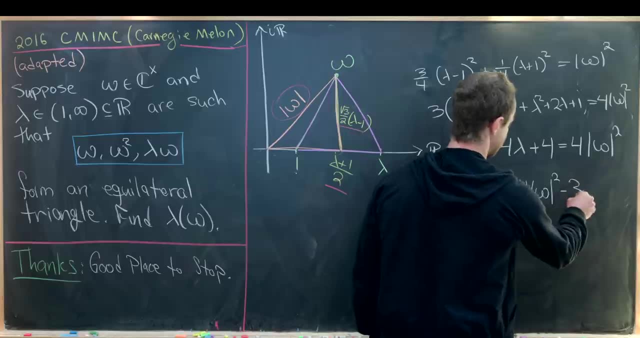 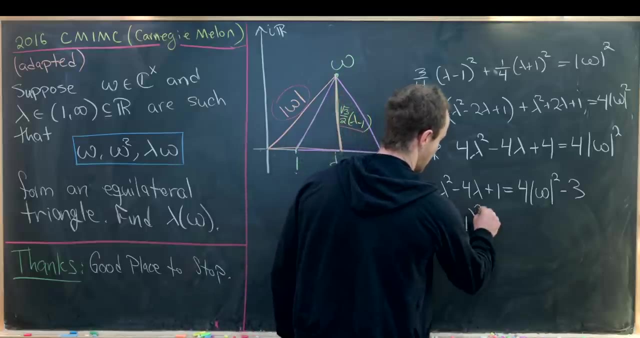 So let's do that. We'll have 4 lambda squared minus 4 lambda plus 1 equals 4 times the modulus of omega squared minus 3.. Then this factors like 2 lambda minus 1, quantity squared equals 4 times omega squared minus 3.. 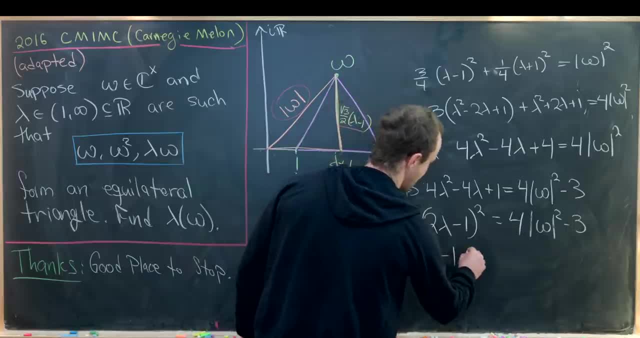 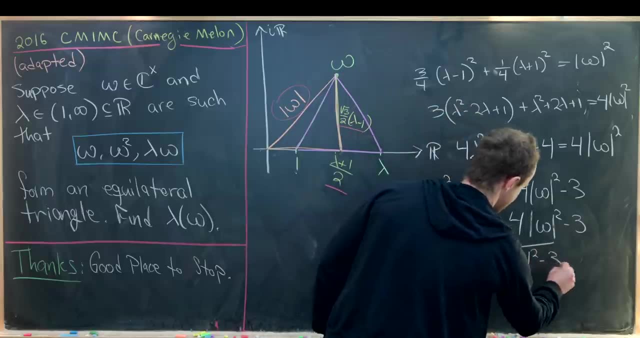 We can take the square root of both sides. We have 2 lambda minus 1. Equals the square root of 4 times omega squared minus 3.. Here we'll take the positive square root, Given that we want lambda to be positive and bigger than 1..